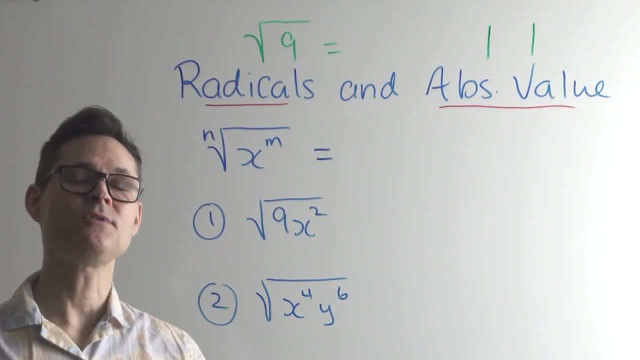 principal square root, or the positive square root. In fact, if you put that into the calculator, it's not going to tell you negative three, It's going to tell you positive three. So the answer is positive. Okay, and that has to do with the definition of that square root symbol On its own. 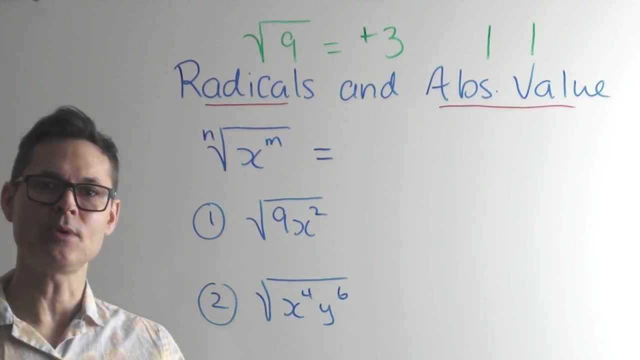 it means: what's the positive square root, what's the number that, when multiplied by itself, will give the number under the radical, the nine? Now we know that negative three times negative three is also nine, but it doesn't want the negative case, So we're going to take the negative three. 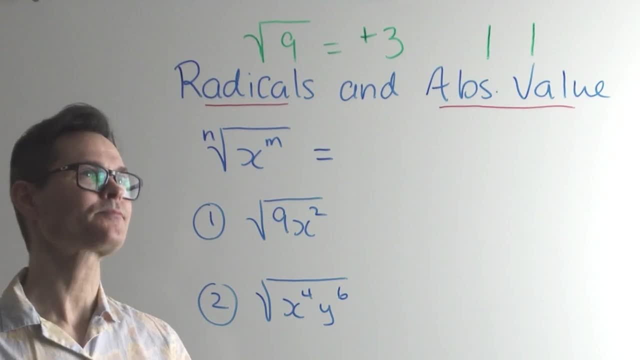 It wants the positive case. Okay, So this is true whenever the index here is, even Now. in this case, it's square root. But this, what I'm about to tell you, is, any case, where the index is even okay, where n is, even where n is, even If n is not even, then what we're about to talk about? 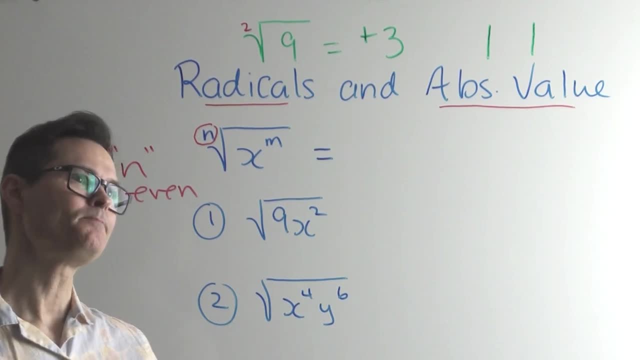 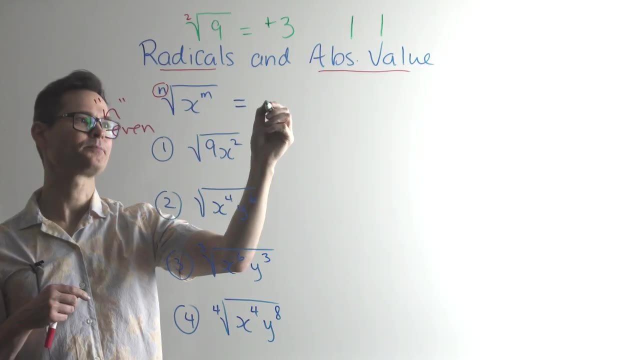 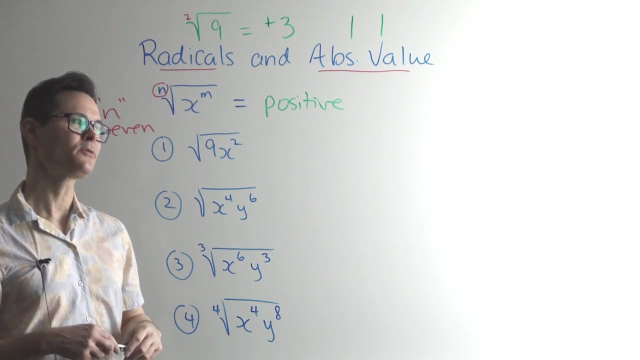 doesn't hold. Okay, it has to be even, And so the idea here is that when n is even, the answer that we place has to be positive, Because it wants the principal nth root or the positive nth root. And again, this is only true when n is even two, four, six, eight and so on. 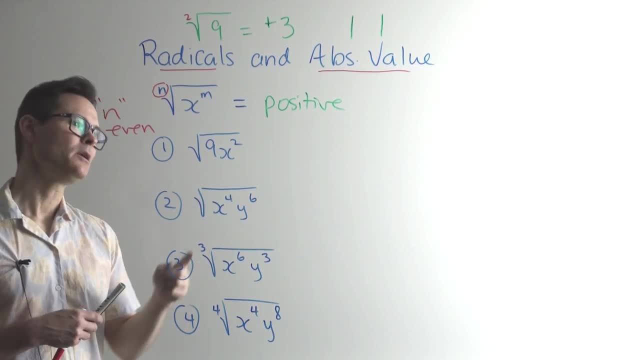 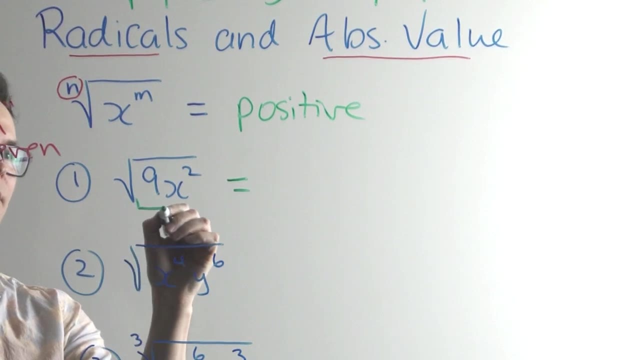 So let's take a look at some examples that make this point. Now, here's the square root of nine: x squared. So when we do this, most of you are going to know that you go through and you say what's the square root of nine And you say the answer is three. 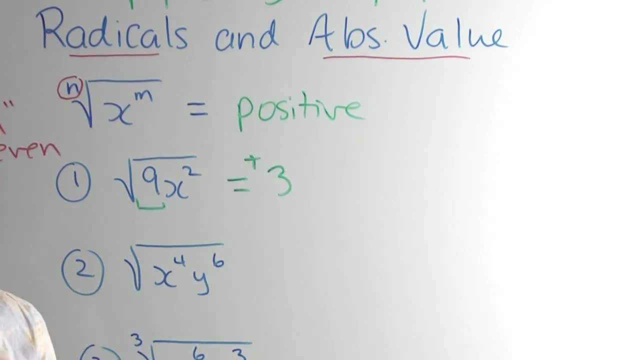 Negative three, Because we have to ensure that the answer is positive. Okay, And then we say: the square root of x squared? Well, look, the index is two. So what I could do here is say the answer is x. This here gets divided by that, So two over two. Or the square root of x squared is: 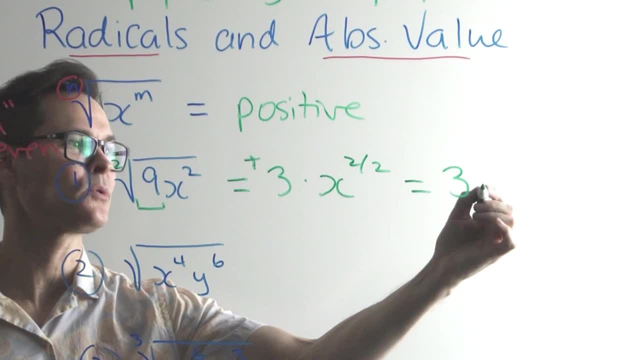 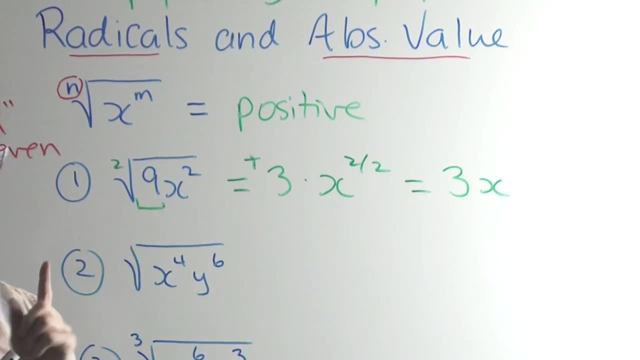 x right, And you would then say that the answer is three x, x to the one. Now you have to be careful here Because, remember, this has to balance for anything. So if you're going to put any possible input on x, if I was to put a square box around the x, call it the x box. if I was, 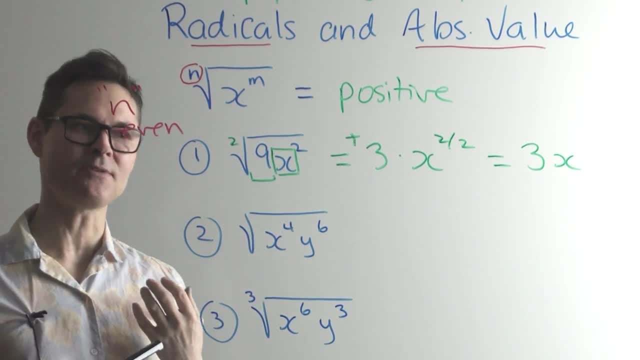 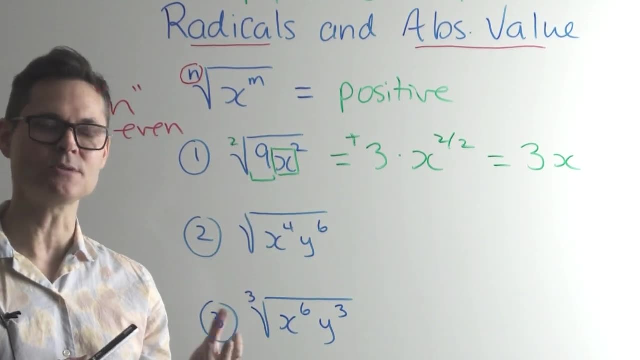 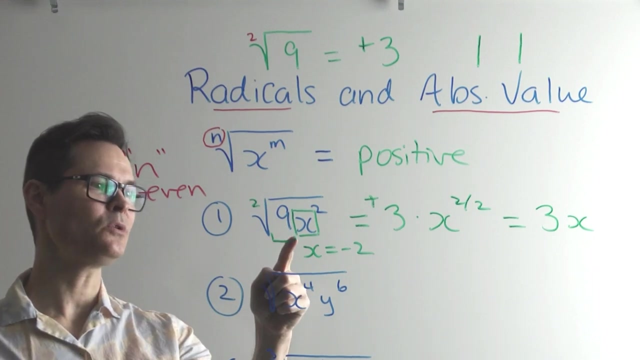 to type in a number here that's negative. it will take the negative value, Because look what's happening- You're squaring the number before you square root it. So this actually accepts negative values. Now. so in other words, say x is equal to negative two. Well, negative two is negative two. 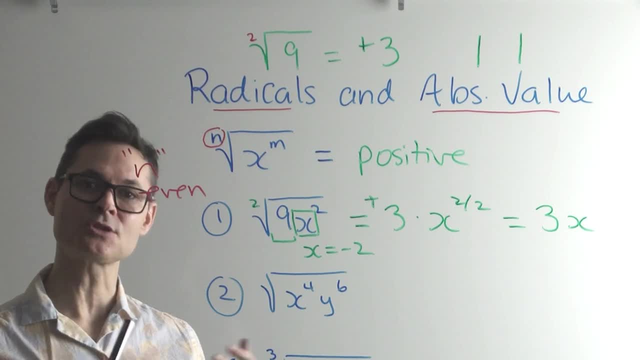 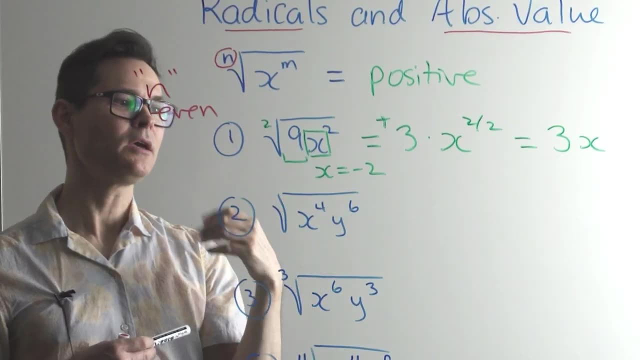 squared, which is four, Four times nine is 36.. So negative two is negative two squared which is 36.. The square root of 36 is six. So this original question, not simplified- this original blue question, works for negative two. Now, if I put negative two into here, I get an answer of negative. 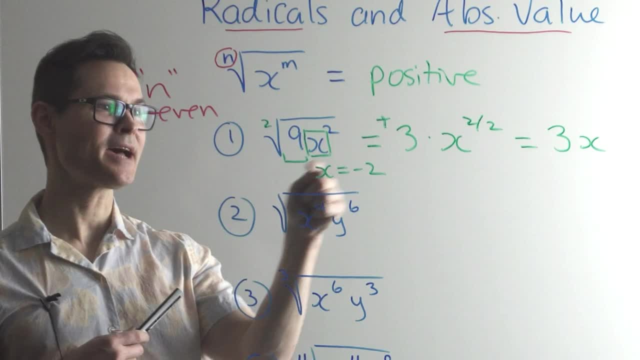 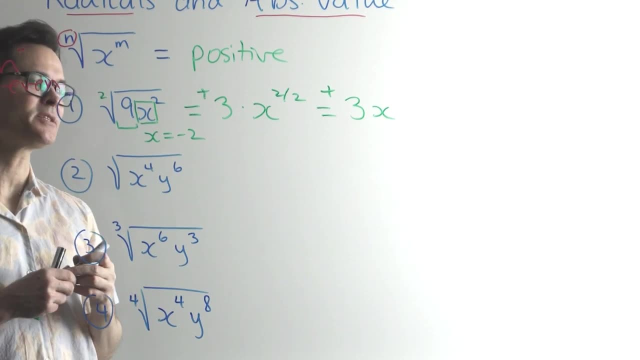 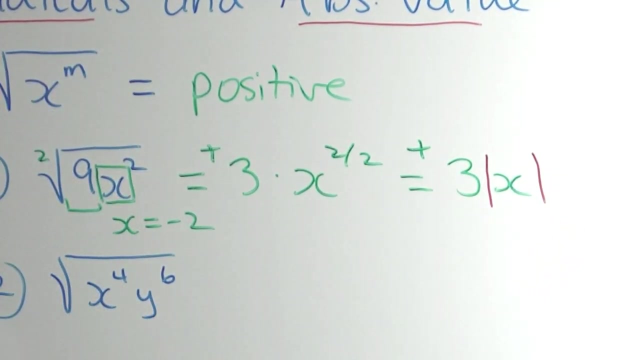 six. Well, that's not balancing right. So this has to be equal to this. Not only that, but we want the positive answer. So in order to ensure that we have a positive answer for x, for cases where x is negative, we have to put an absolute value set of brackets around the x box. So 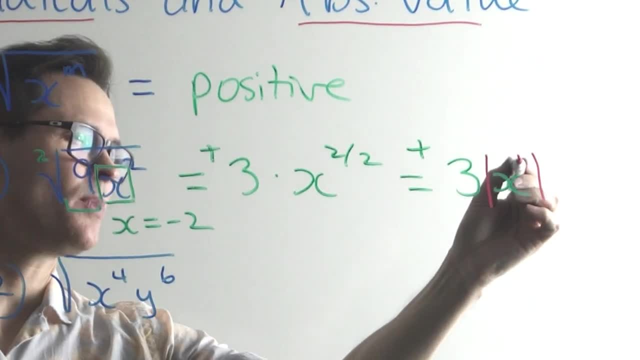 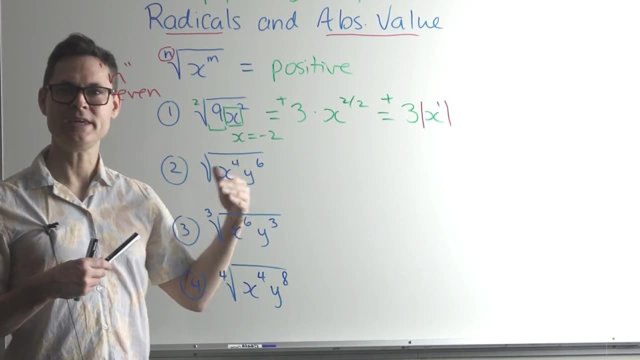 let's look at this next question. This only is true when the exponent on the answer is odd. Okay, so one, three, five and so on. Let's take a look at this next one here. If I was to now, this is: 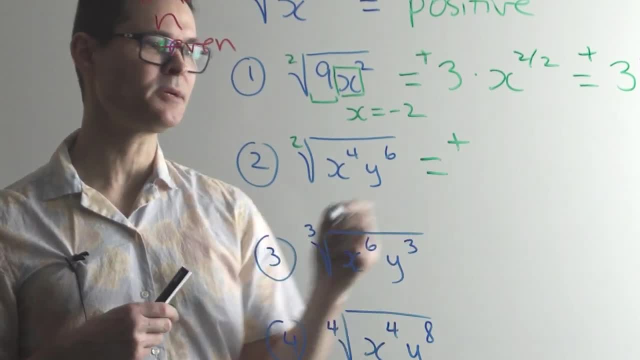 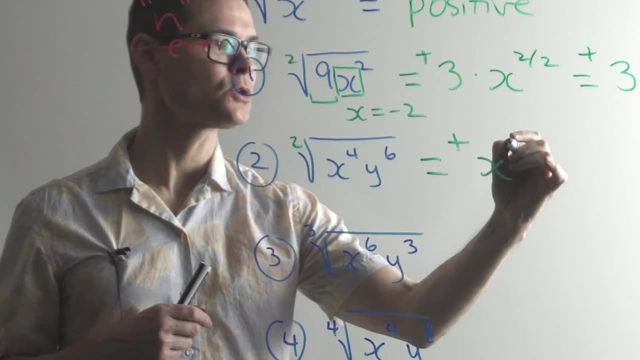 square root land again. So to build my answer, which I want to be positive, right, because I'm asking for the principal square root, that's going to be x, four over two, So four divided by two, And then I'm going to have to divide by two. So I'm going to have to divide by two And then I'm 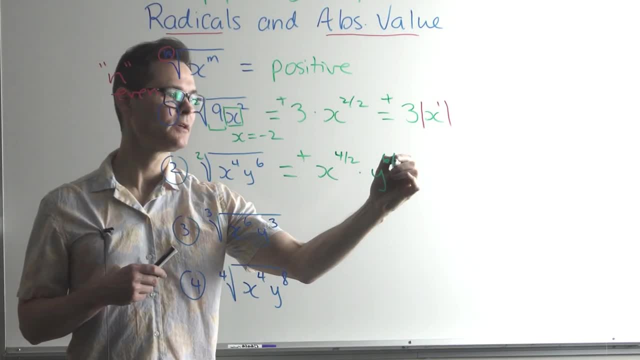 going to have to divide by two, And then I'm going to have to divide by two, And then I'm going to have to divide by two. Okay, now break this down. So that's going to be equal to well, x squared x. 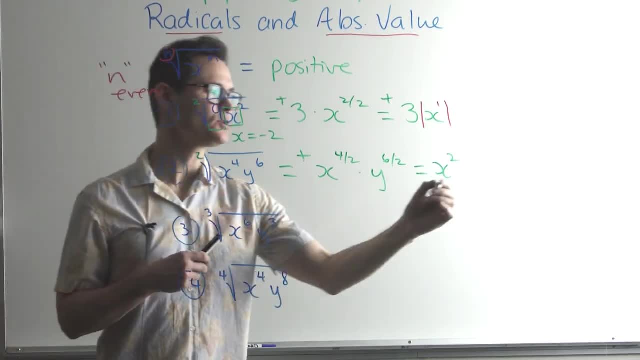 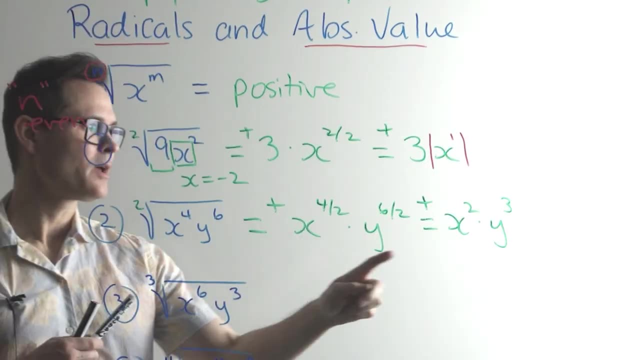 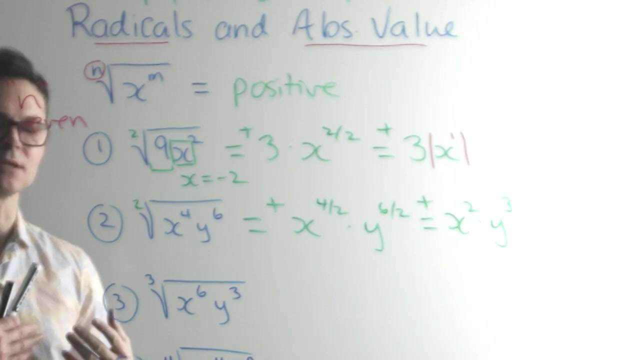 squared And then the y to the six over two is going to be y to the three. Now just double check, make sure that the answer is going to be positive. The this here is okay. x is okay because, look, x squared. the square is going to ensure that the answer stays positive. But look here, y is being 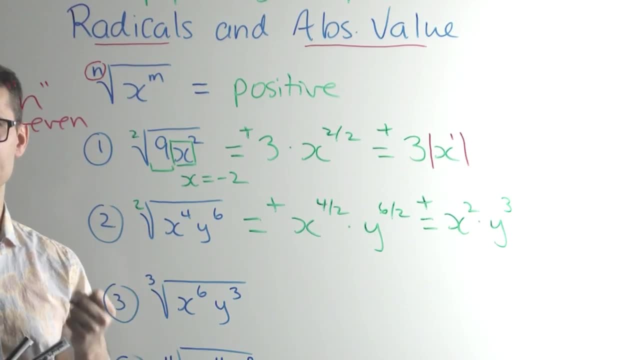 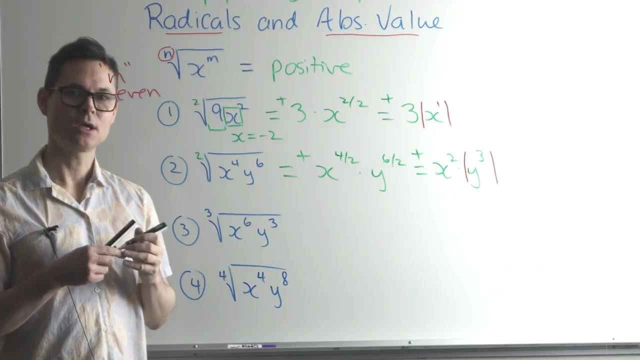 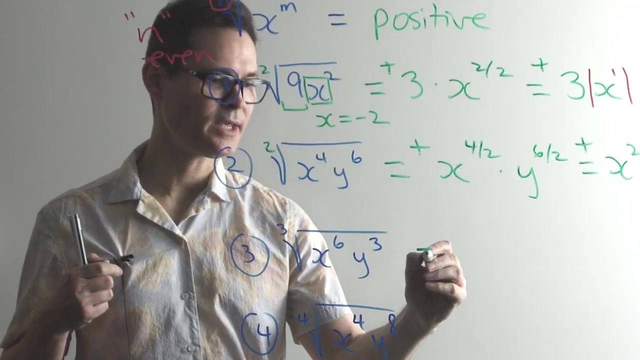 cubed, And so the cube doesn't guarantee that the answer stays positive. So in this case you have to put absolute value around the y. you can put it around the x, but it's redundant, it's not needed. Let's take a look at the next one here. So we get into a little bit of a role here. Check here. 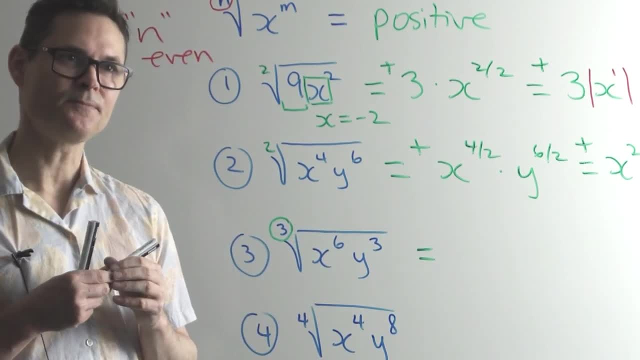 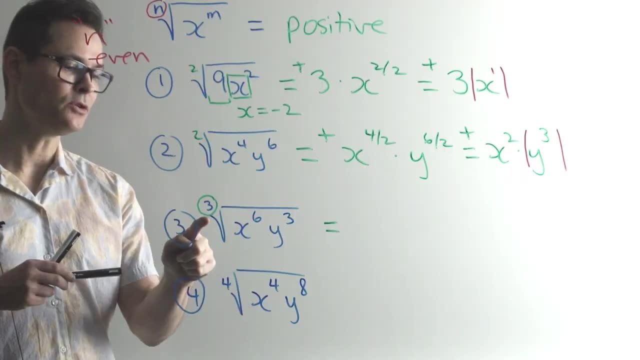 notice now. the outside index is three. this rule is only applicable when n is even. So in this case, here we don't use absolute value, So we're going to have to divide by two, So we're going to have to use absolute value. brackets- you don't need them for odd indices, So here the answer would be x six. 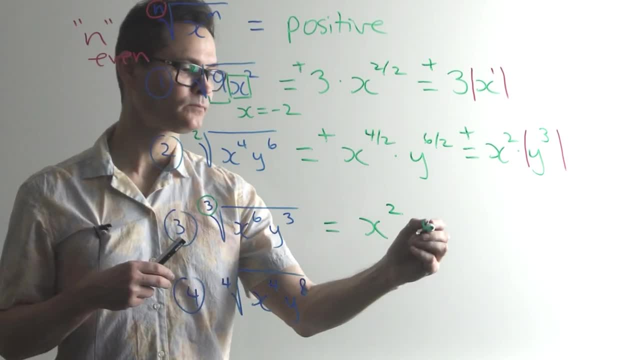 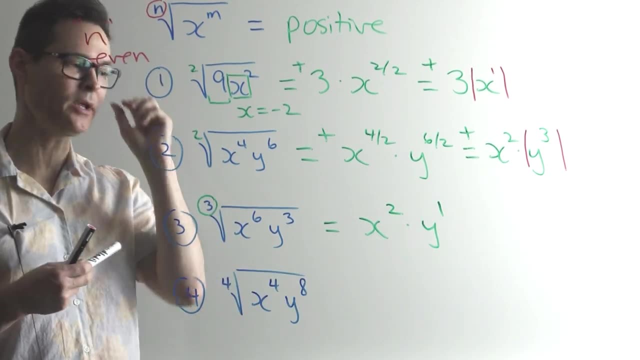 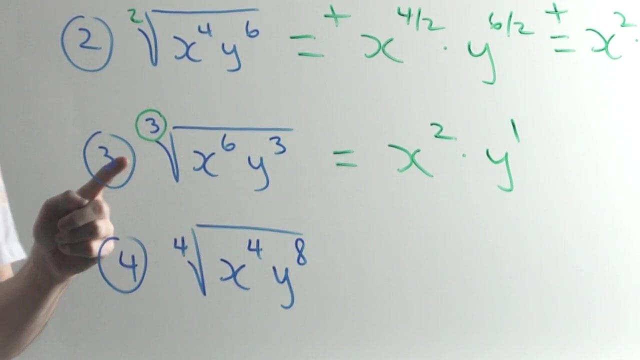 divided by three, which is two, And then y three divided by three, which is one. Now, even though y is being raised to an odd exponent, you don't want to put the absolute value here, Because when you take the cube root of a number you can get a negative value. So we don't try to ensure positiveness. 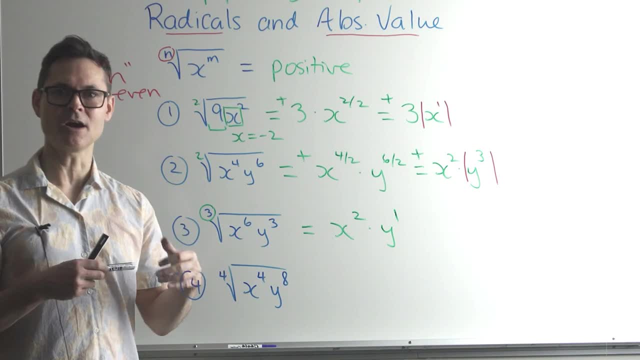 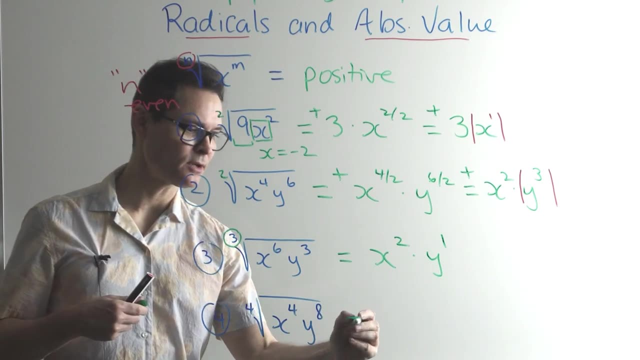 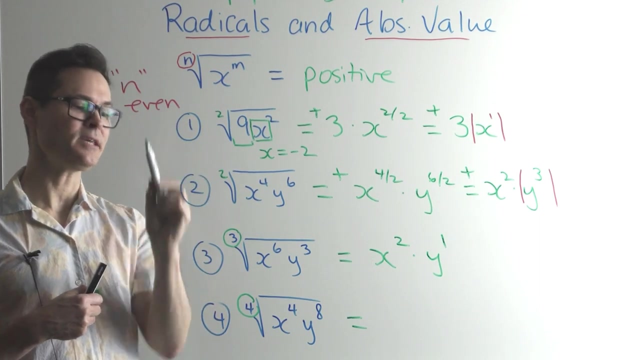 in our answer for for indices that are odd. okay, so you leave it just like that. and now the last one here. this one looks like it could be important to consider because, look, the index is 4. so if the index is 4, again, n is even, 4 is even, so we we tread carefully here. so X, 4 over. 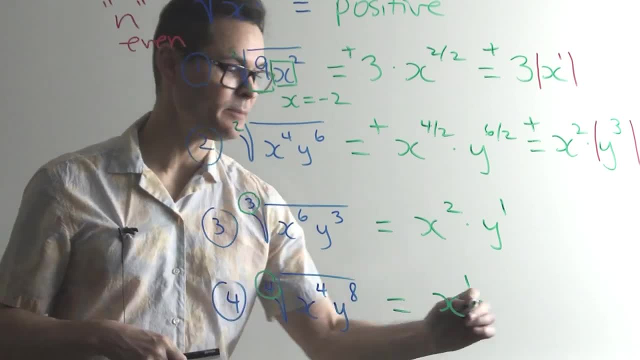 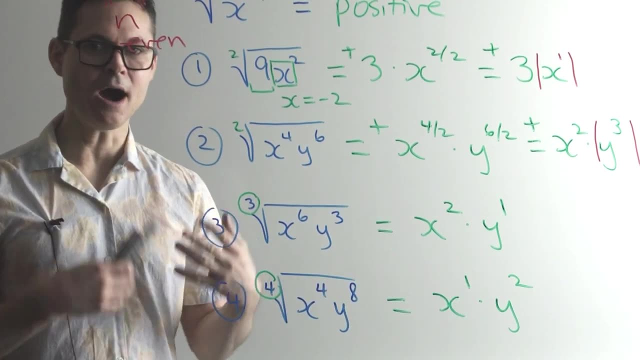 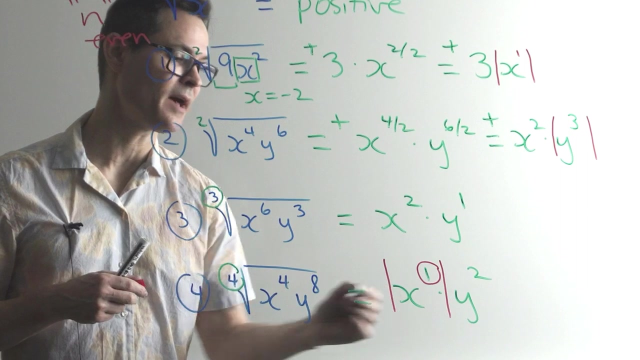 4 is 1 and Y to the 8. 8 divided by 4 is 2. so in this case we check our exponents and the answer and if either of them are odd- and in this case it is see, that's a one- then you have to install your absolute value brackets. okay, I don't. 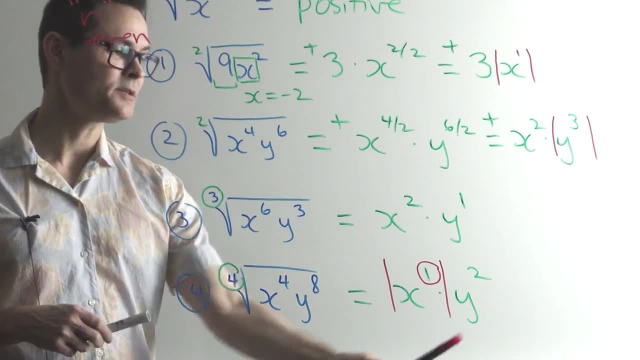 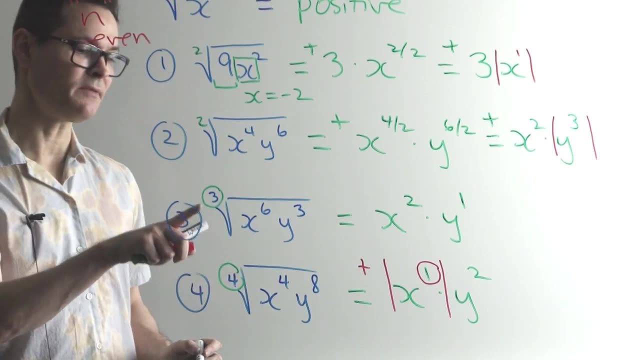 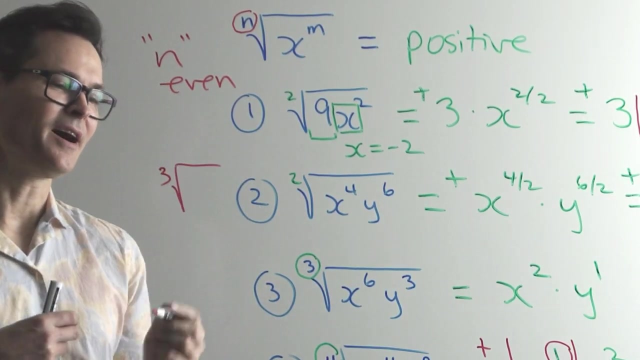 need to worry about the Y, because the square on the Y is going to ensure that the answer stays positive. remember: when the index is even, you want a positive answer. when the index is odd, the answer can be negative. right, don't forget the cube root of negative.